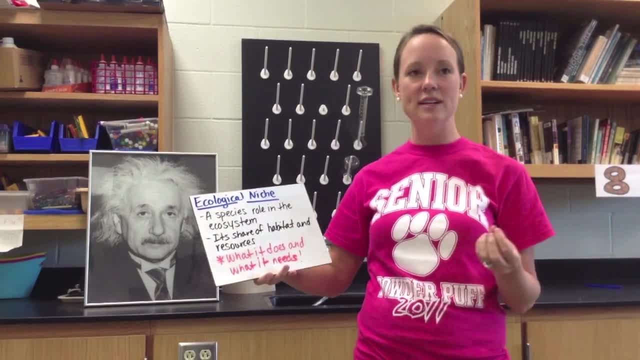 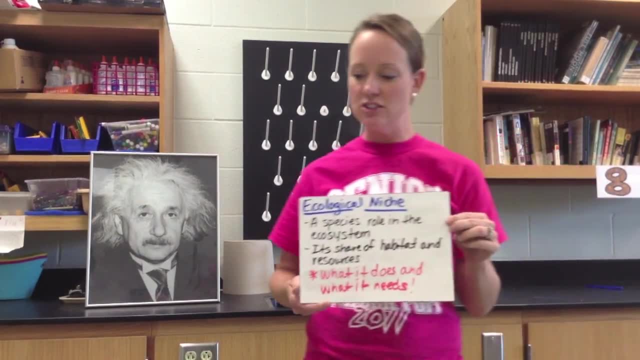 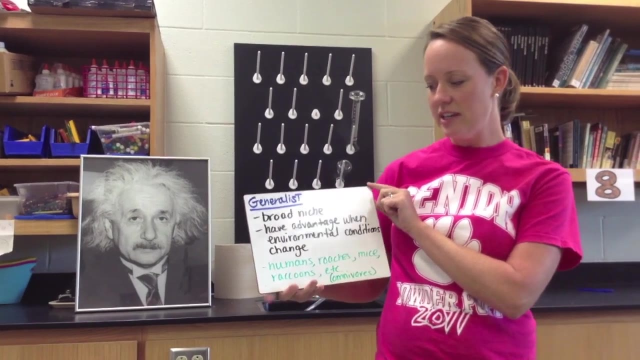 another way that we can say. that is what the organism does and what resources it needs. And the organism's niche determines if it is a generalist or a specialist species. If it's a generalist, that means it has a broad niche So it can use a wide variety of resources. it can eat a variety of foods, So these are usually going to be your omnivores. They can survive off eating plants or animals. They can tolerate a wide range of environmental conditions, So they can survive in different climates as well. So these types of species- 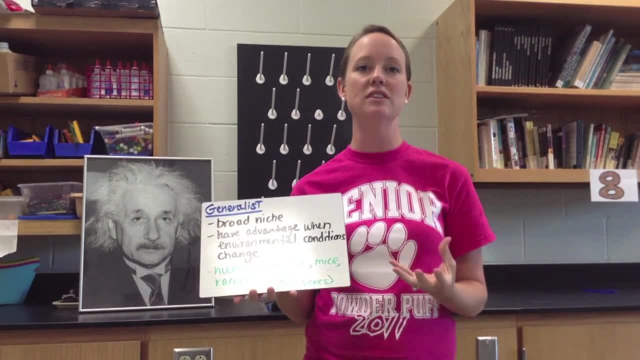 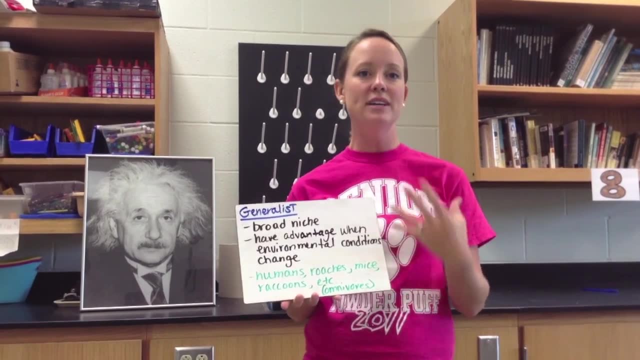 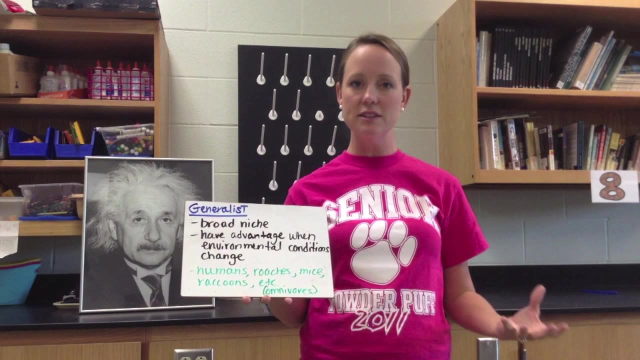 are going to have an advantage when there is a change in the environment. If there's a catastrophe in an ecosystem, they're going to be those that are most likely to survive, because they can live in different types of conditions. Some examples: humans. We can move from place to place. We can live in different biomes. We can eat different. foods. Roaches tend to survive everything. Mice raccoons- raccoons will eat just about anything. If a species has a narrow niche, it is known as a specialist. They tend to live in only one type of habitat. They have a narrow range of climate and other environmental conditions. 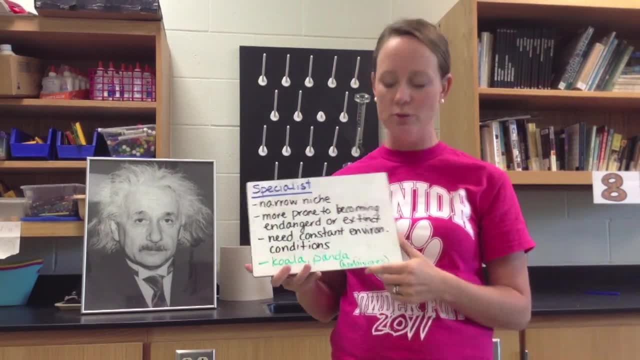 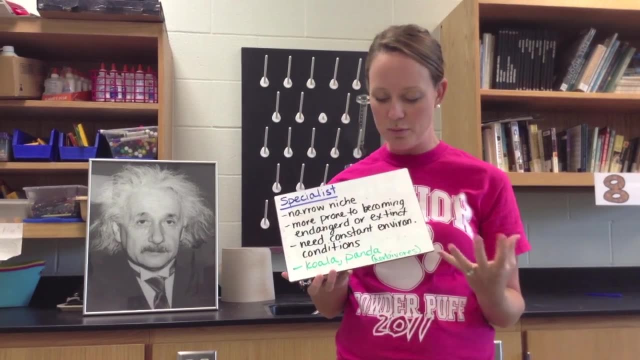 They can only eat one or two types of food, So usually these are going to be herbivores. An example would be the koala. A koala can only eat eucalyptus. They depend on one plant. Same thing with the giant panda: They only eat bamboo. So these are the types of organisms. 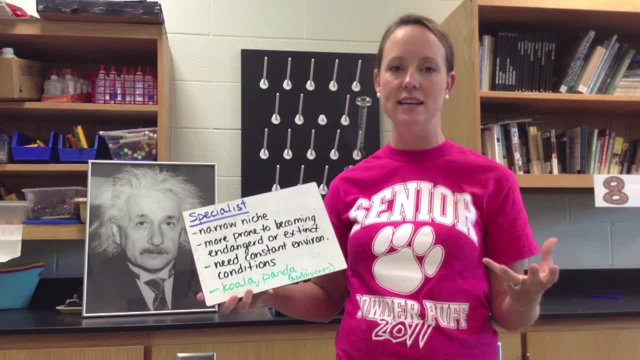 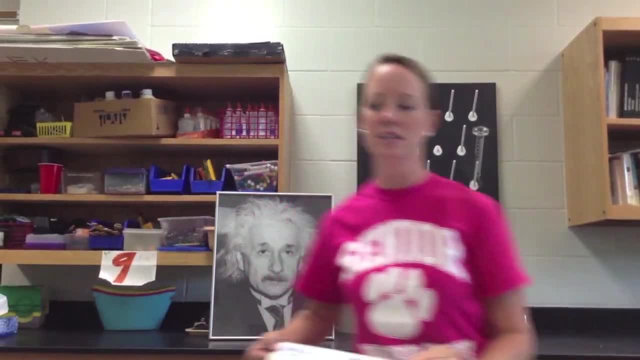 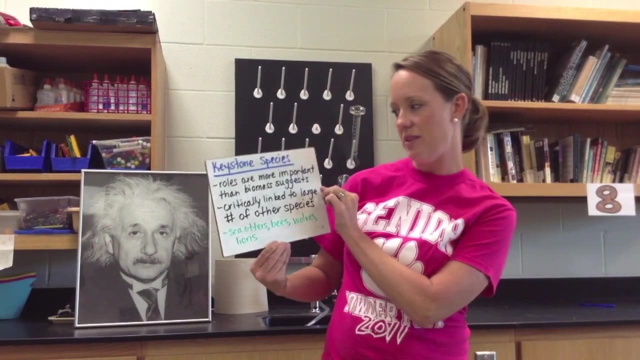 that are going to be more prone to being endangered or becoming extinct And they cannot adapt to changing environmental conditions. Other classifications of species in an ecosystem. If an organism has a pivotal role in the ecosystem, that that is more important than their size suggests, they're known as a keystone species And usually 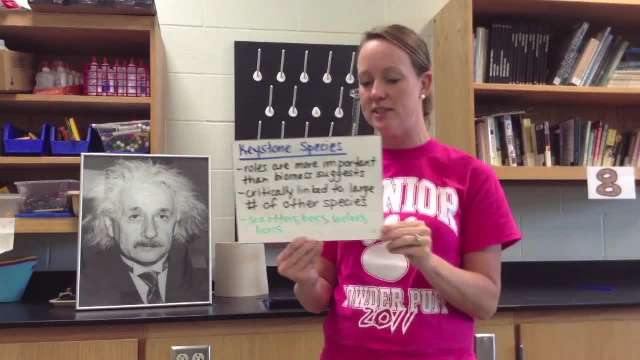 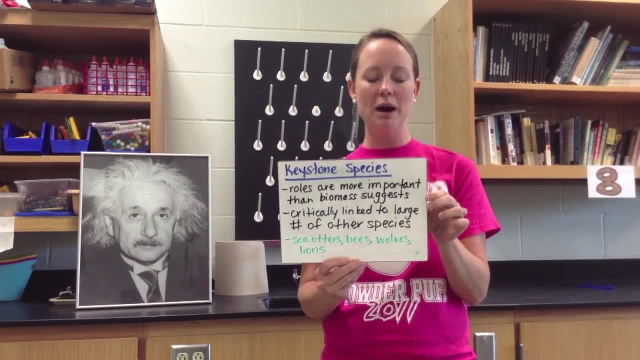 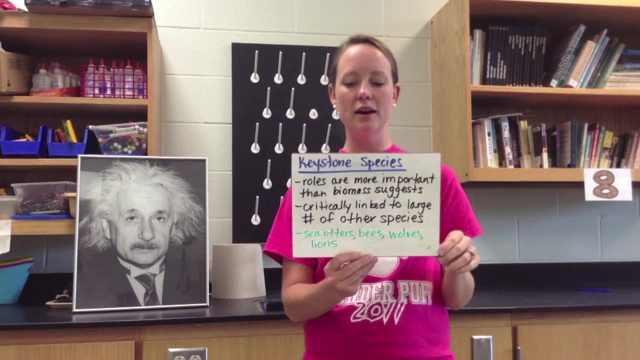 they're going to be critically linked to a large number of species in the ecosystem. So if something happens to one of these organisms, usually that can lead to population crashes or even extinction of other organisms. One example of a keystone species would be butterflies. 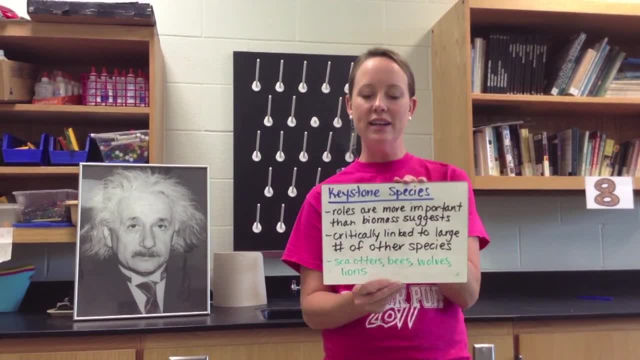 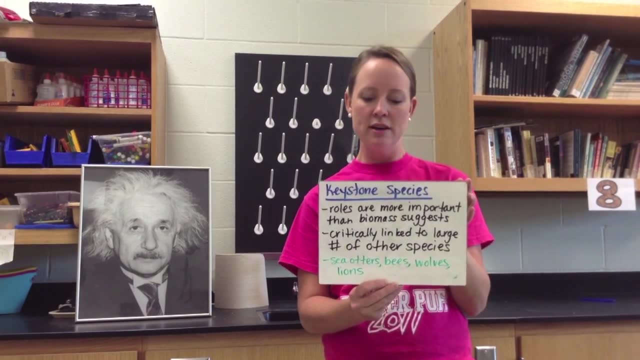 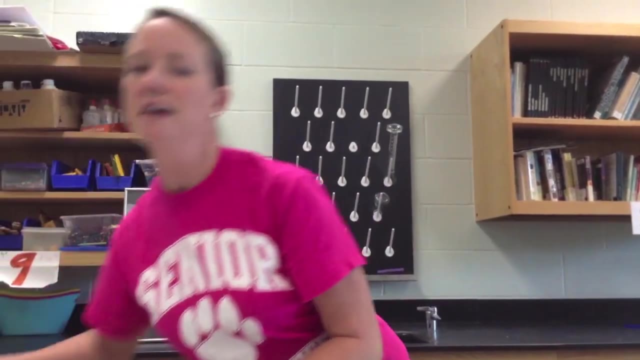 or bees or hummingbirds that are important in pollination of flowering plants. They can be considered a keystone species. Also, a top predator can be considered a keystone species. They help regulate the population of the species that they feed on. A foundation species is a type of keystone species. They play an important role in creating 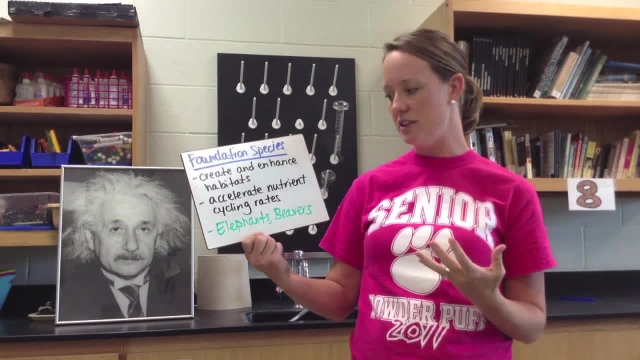 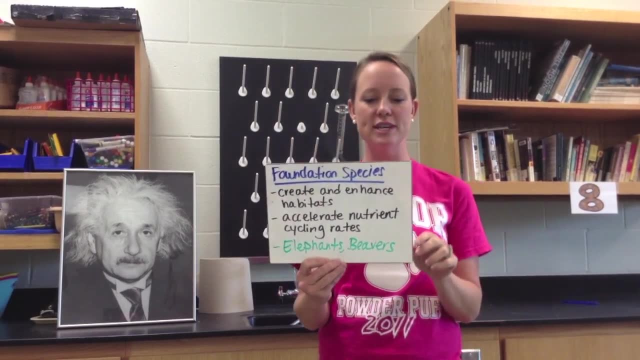 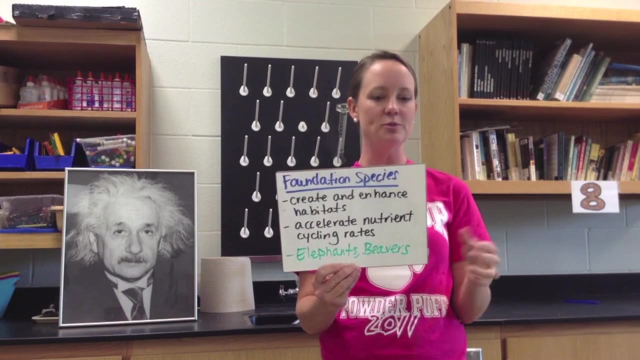 and enhancing a habitat. They can also accelerate the nutrient cycling rates. An elephant is an example. What elephants do is they'll push over, break or uproot trees And they'll create openings in the grasslands and woodlands in Africa so that organisms like antelopes 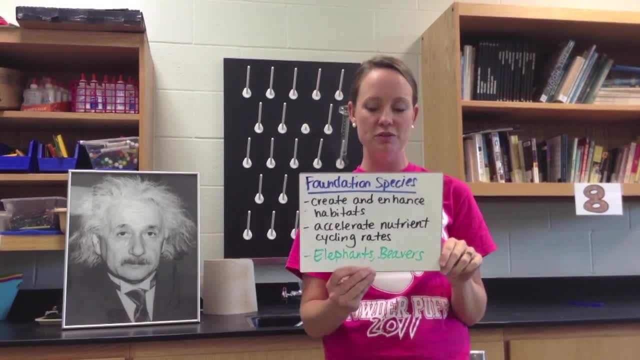 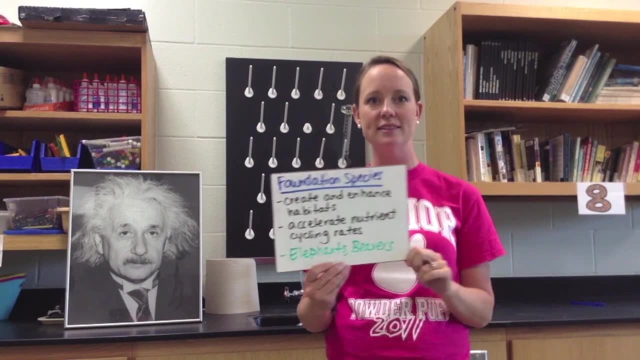 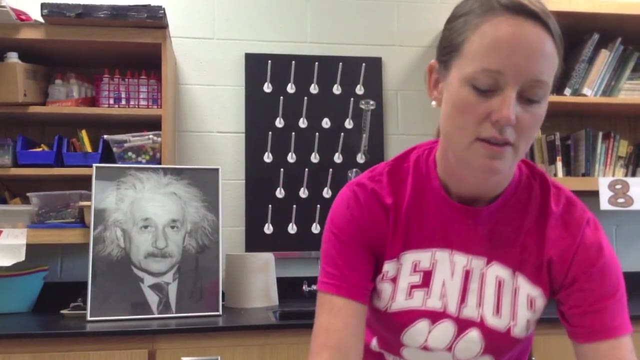 can eat on the grasses and other plants that benefit from the removal of trees. Beavers would be another example. They are engineers. They build dams, which creates ponds and wetlands, And it almost creates a new habitat for other organisms. An indicator species is a species. 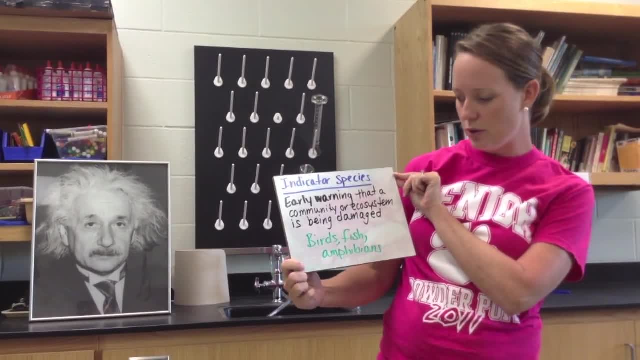 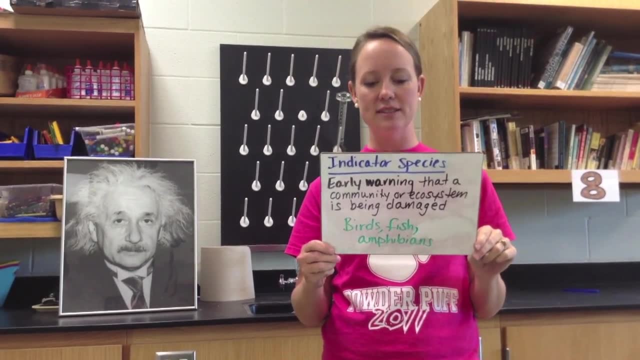 that serves as an early warning in a climate. An indicator species is a species that is an early warning in a community or ecosystem if something is happening. Birds, fish and amphibians are all good examples of indicators because they respond very quickly to environmental. 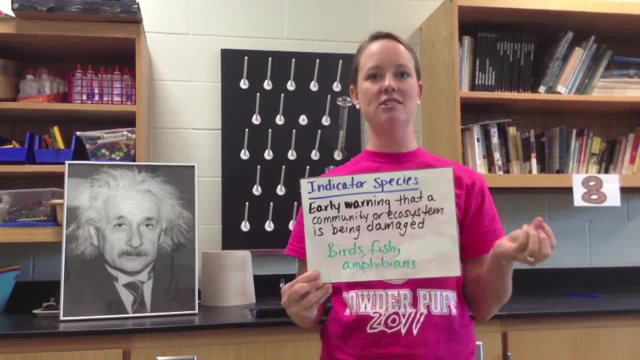 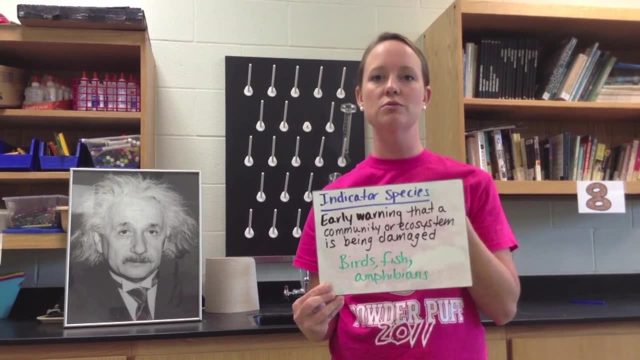 change. One example: coal miners used to take canaries into the mines with them, And when the canary died, the miners knew that they had to get out quick because the birds were going to react to change in the gases or lack of oxygen much faster than a miner would. 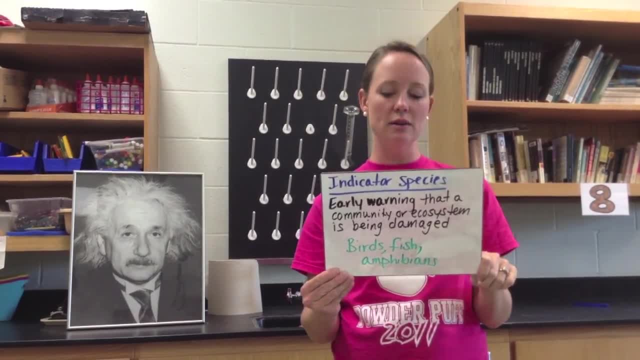 Fish are good examples. Trout, for example, is a good example of an indicator species. You can find a lot of them. I'm going to show you one. Trout is one that requires clean water and high levels of dissolved oxygen. So if there's an organic pollutant dissolved, oxygen levels drop and you start seeing an absence of the trout Species that normally live and thrive in an ecosystem are called native species, And those species that are introduced either accidentally on purpose by humans or migrate into an area are known as non-native. You'll also see them called exotic or exotic, which means that they are 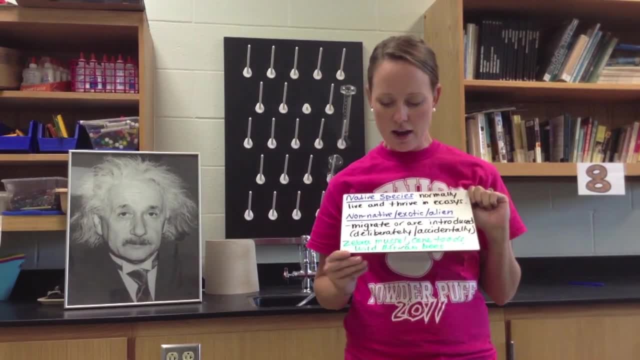 not considered native species. So now you can see all these species that are introduced, exotic or alien species. Some of the examples we'll look at in case studies later on this year: the zebra mussels in the Great Lakes. the wild African bees. 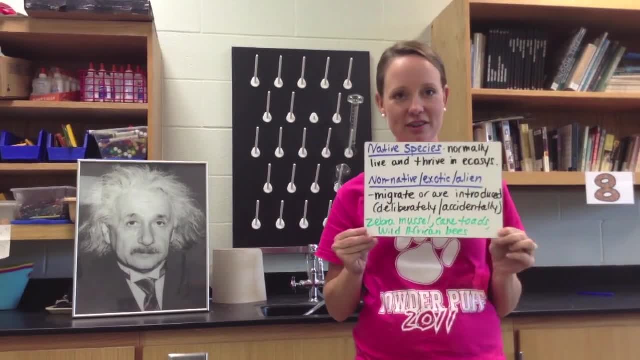 and then my favorite, which you'll soon come to find out: why are the cane toads?